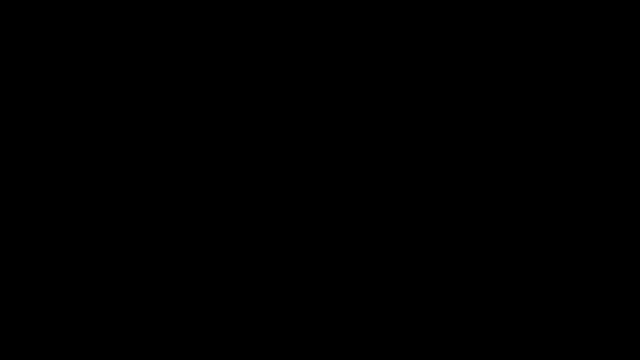 In this video we're going to talk about the differences between acute angles, right angles, obtuse angles and straight angles, And we're also going to go over some common geometry problems associated with right angles and things like that. So what exactly is an acute angle? 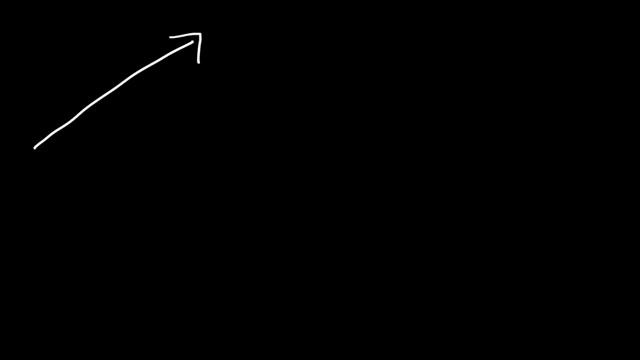 So first let's start with a picture. An acute angle is an angle that is less than 90 degrees. So let's say X represents the angle, So X is going to be less than 90 degrees. Now the next angle that we need to talk about is the right angle. 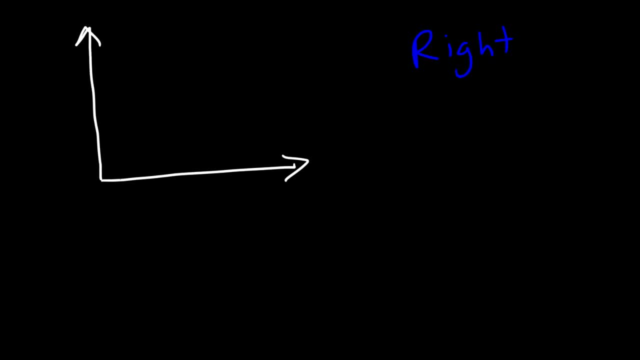 A right angle has an angle of 90 degrees. Typically, you'll see, You'll see a box right next to the vertex. So X is exactly 90.. The next angle you need to be familiar with is an obtuse angle. An obtuse angle is a relatively large angle. 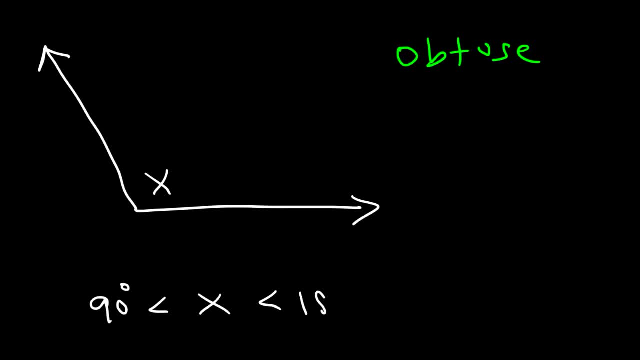 The angle is greater than 90, but less than 180. So that is an obtuse angle. And finally, A straight angle. A straight angle is basically the angle of a straight line, And a straight line always has a measure of 180 degrees. 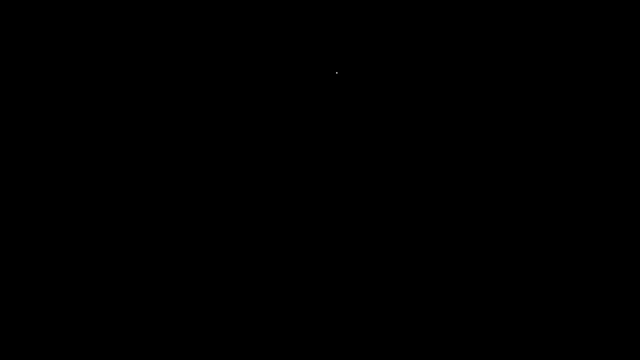 So that's a straight angle. A full circle is always 360 degrees, But half a circle is 180.. So notice that if you draw a straight line, the angle that forms is basically in the shape of a semi-circle, That's 180.. 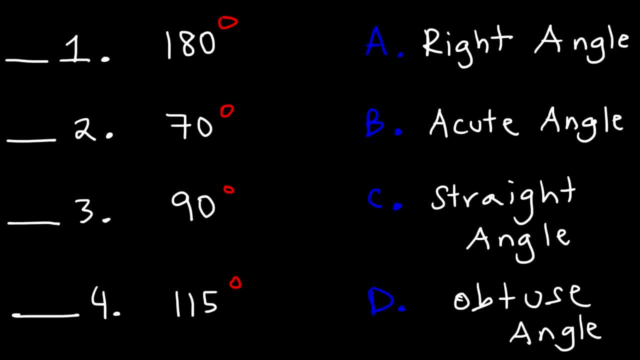 So here is a simple matching quiz. Feel free to pause the video and classify each angle as a right angle, acute angle, straight angle or an obtuse angle. Now, this is pretty much an easy quiz, so feel free to do it if you want to. 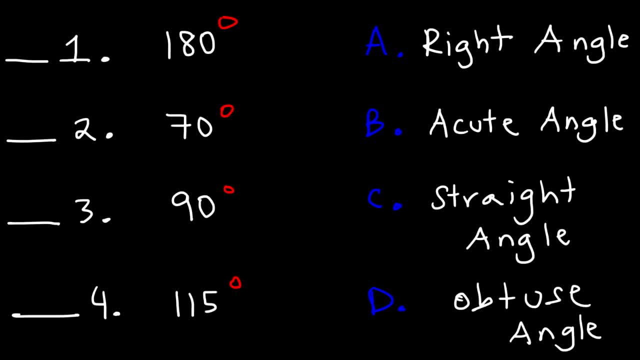 So let's start with number one. So if we have an angle of 180 degrees, which answer choice- does that correspond to? Is that a right angle, Is it acute? Is it a straight angle Or an obtuse angle? If it's exactly 180, then it is a straight angle. 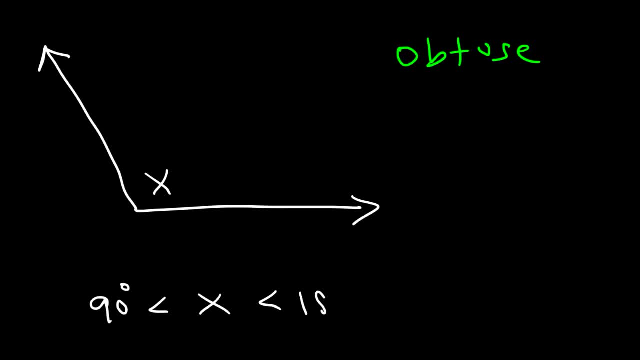 The angle is greater than 90, but less than 180. So that is an obtuse angle. And finally, A straight angle. A straight angle is basically the angle of a straight line, And a straight line always has a measure of 180 degrees. 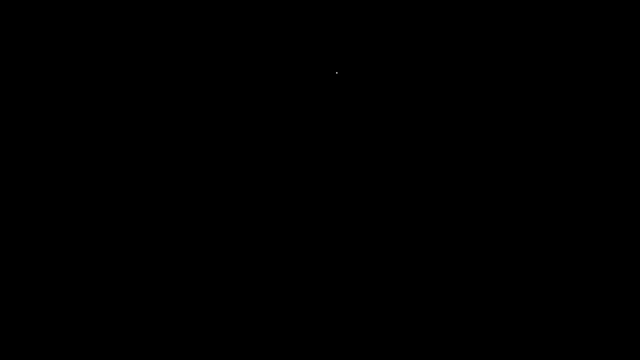 So that's a straight angle. A full circle is always 360 degrees, But half a circle is 180.. So notice that if you draw a straight line, the angle that forms is basically in the shape of a semi-circle, That's 180.. 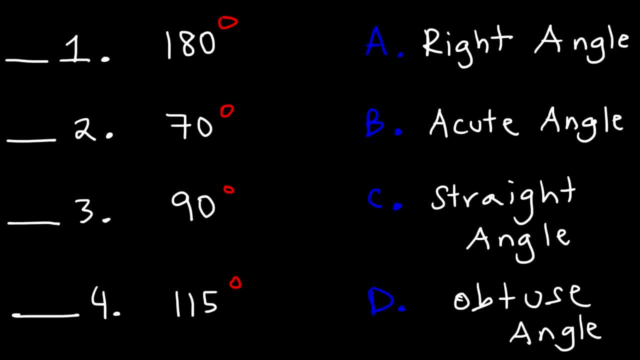 So here is a simple matching quiz. Feel free to pause the video and classify each angle as a right angle, acute angle, straight angle or an obtuse angle. Now, this is pretty much an easy quiz, so feel free to do it if you want to. 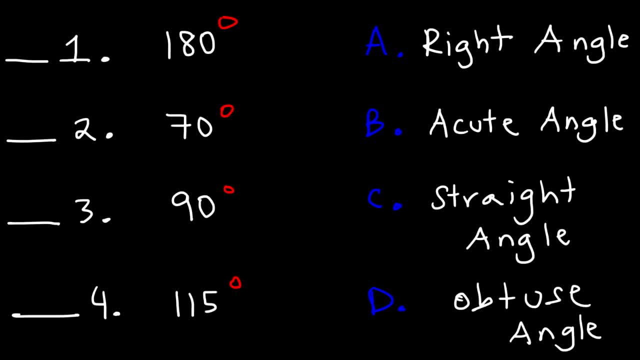 So let's start with number one. So if we have an angle of 180 degrees, which answer choice- does that correspond to? Is that a right angle, Is it acute? Is it a straight angle Or an obtuse angle? If it's exactly 180, then it is a straight angle. 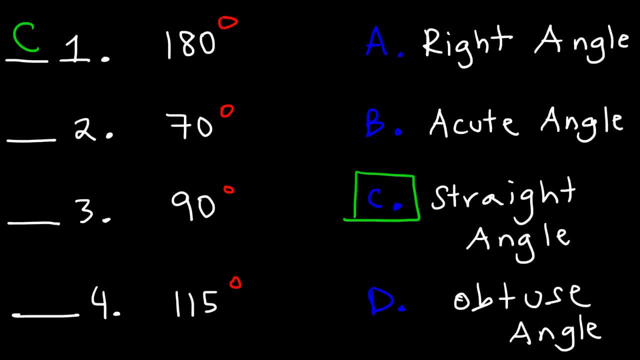 So therefore, number one is answer choice C. Number two: An angle of 70 degrees corresponds to which answer. Number two represents answer choice B. An acute angle is any angle that is less than 90.. So if it's 50.. 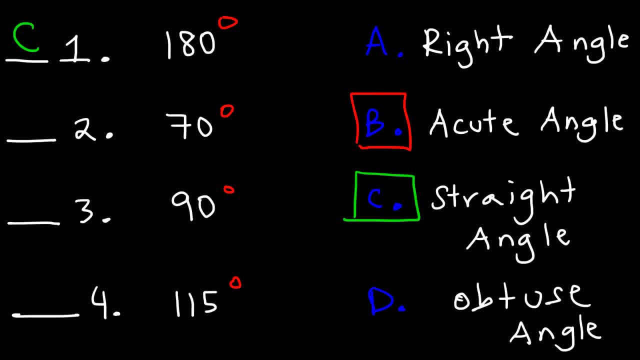 70. 45. Those are all less than 90, so number two represents an acute angle. Number three is exactly 90,, which is a right angle. So number three is the answer, choice A. And finally, number four by default has to be the obtuse angle. 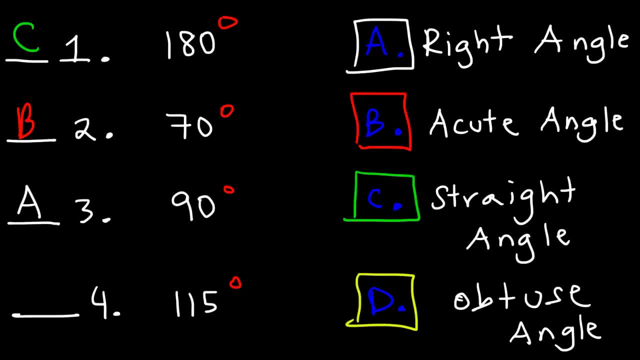 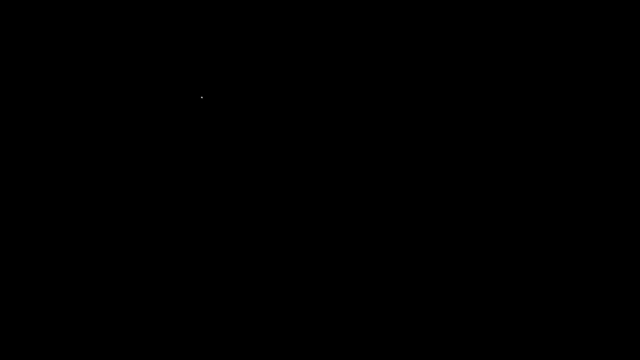 An obtuse angle is between 90 and 180.. It's greater than 90, so 90.1 would be an obtuse angle, But it's less than 180.. So 179 is an obtuse angle And therefore 115 is also obtuse. 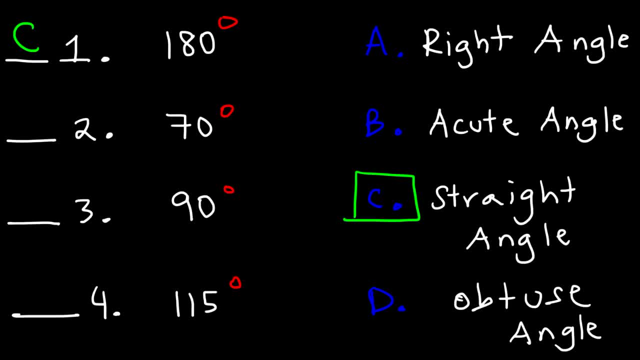 So therefore, number one is answer choice C. Number two: An angle of 70 degrees corresponds to which answer. Number two represents answer choice B. An acute angle is any angle that is less than 90.. So if it's 50,, 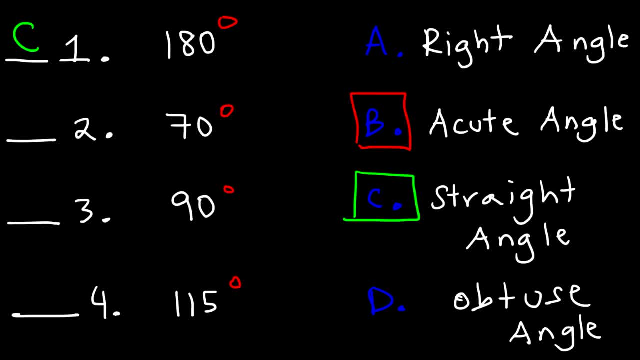 70,, 45,. those are all less than 90. So number two represents an acute angle. Number three is exactly 90,, which is a right angle. So number three is the answer choice A. And finally, number four by default has to be the obtuse angle. 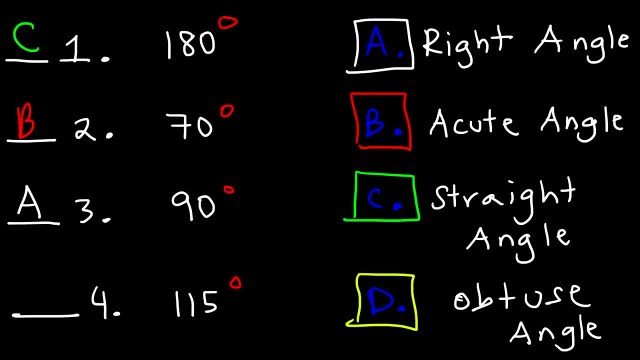 An obtuse angle is between 90 and 180.. It's greater than 90. So 90.1 would be an obtuse angle, But it's less than 180.. So 179 is an obtuse angle And therefore 115 is also obtuse. 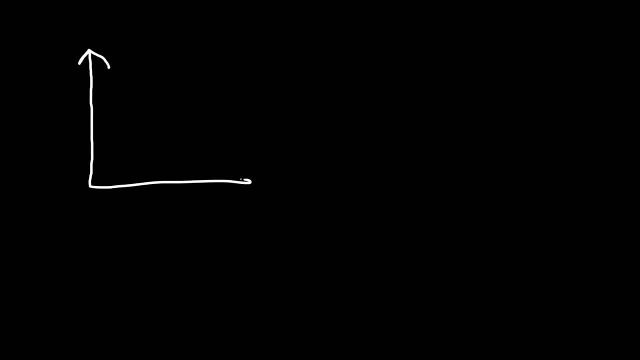 Now let's work on an example problem. So let's say that angle ABC is a right angle. Let's say it's divided into two angles, Not divided evenly. Let's call this angle one And angle two, So angle one is the same as angle ABD. 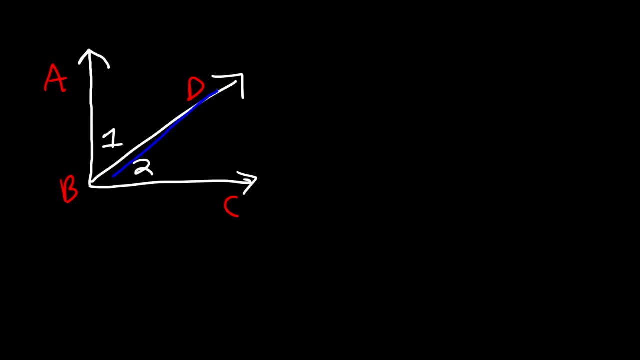 Angle two is equivalent to angle DBC. Now let's say that angle one has a measure of five X plus four And angle two is equal to seven X minus 10.. And keep in mind angle ABC is a right angle, which means that it's equal to 90 degrees. 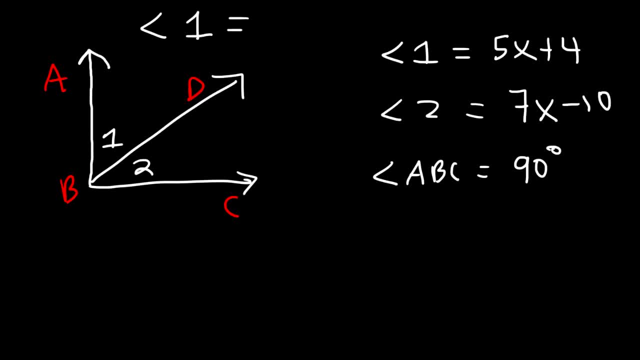 Find the measure of angle one. So feel free to pause the video Now. before we do this problem, I want to give you some examples. So I'm going to draw angle ABC again Now. let's say, if angle one is equal to 40 degrees, 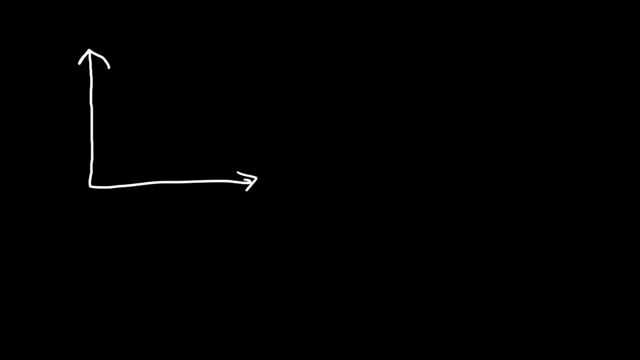 Now let's work on an example problem. So let's say that angle ABC is a right angle. Let's say it's divided into two angles, Not divided evenly. Let's call this angle 1. And angle 2.. So angle 1 is the same as angle ABD. 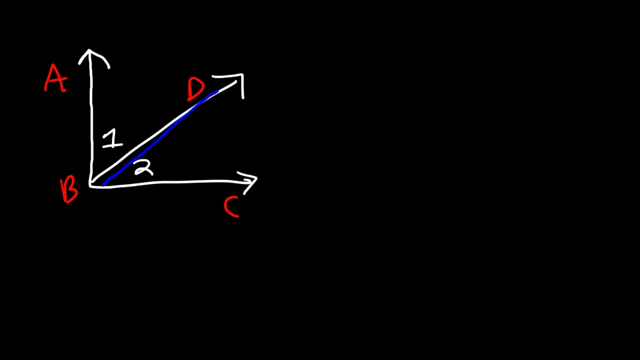 Angle 2 is equivalent to angle DBC. Now let's say that angle 1 has a measure of 5x plus 4.. And angle 2 is equal to 7x minus 10.. And keep in mind, Angle ABC is a right angle, which means that it's equal to 90 degrees. 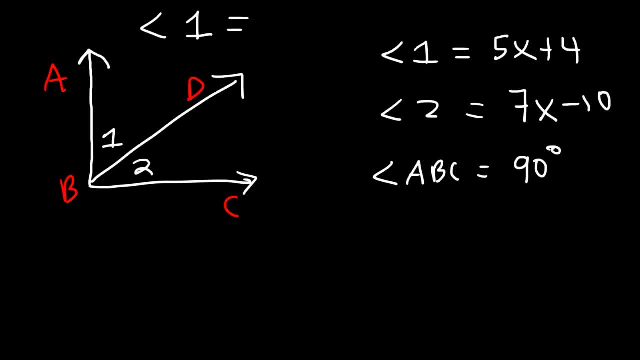 Find the measure of angle 1.. So feel free to pause the video Now, before we do this problem, I want to give you some examples. So I'm going to draw angle ABC again. I'm going to draw angle ABC again. Now, let's say, if angle 1 is equal to 40 degrees, what is the value of angle 2?? 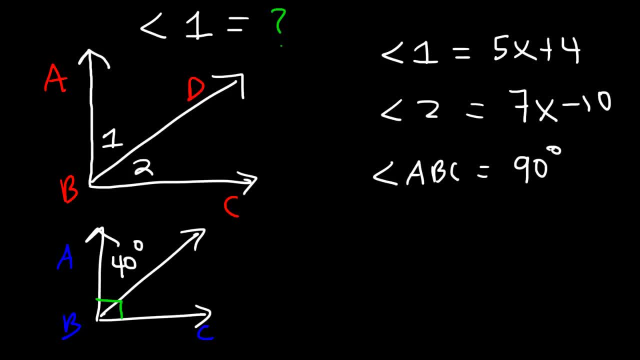 Now keep in mind: ABC is the right angle, which means that it has to add up to 90. So therefore, the value of angle 2 is 50. So these two angles, they have to equal 90, 40 plus 50 is 90.. 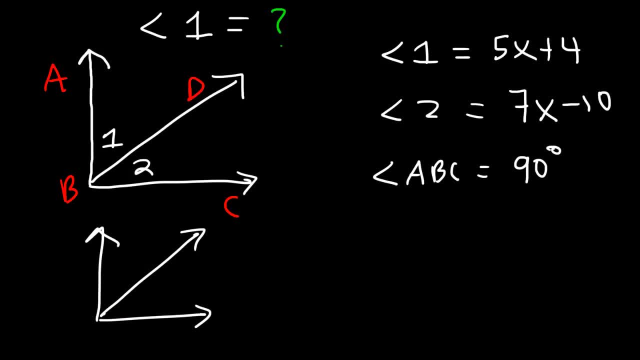 So now let's finish this problem. So we know that angle 1 plus angle 2 has to equal 90. Whenever two angles add up to 90, it's said that those angles are complementary angles. Supplementary angles add up to 180.. 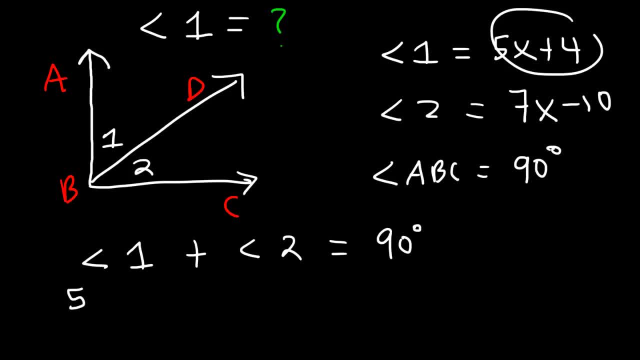 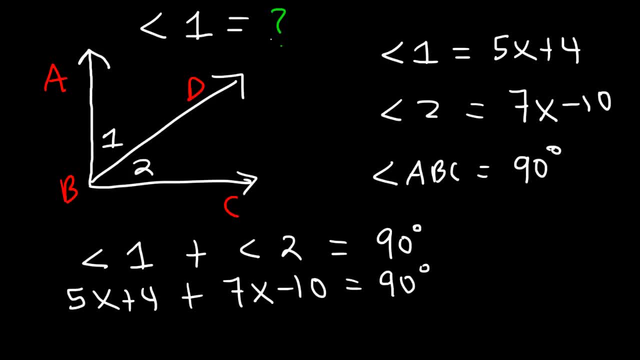 So if we could find the value of x, we could find the measure of angle 1.. Once we have the value of x, all we need to do is plug it in to 5x plus 4, and that's going to give us the measure of angle 1.. 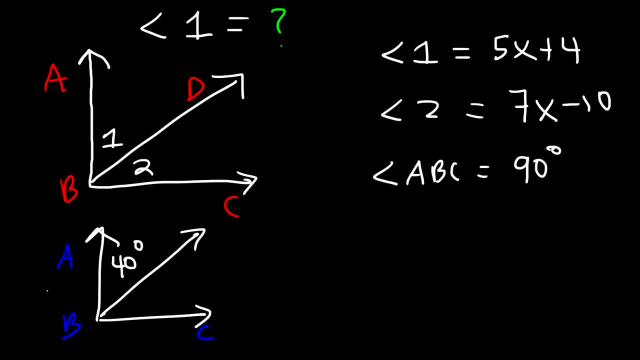 What is the value of angle two? Now, keep in mind: ABC is the right angle, which means that it has to add up to 90. So, therefore, the value of angle two is 50. So these two angles, they have to equal 90.. 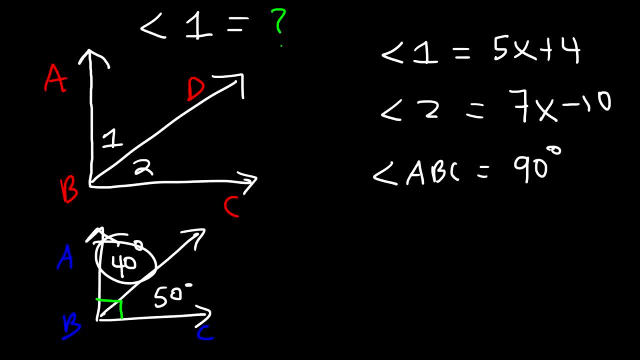 40 plus 50 is 90. So now, let's finish this problem. So now let's finish this problem. So now let's finish this problem. So we know that angle one plus angle two has to equal 90. Whenever two angles add up to 90,. 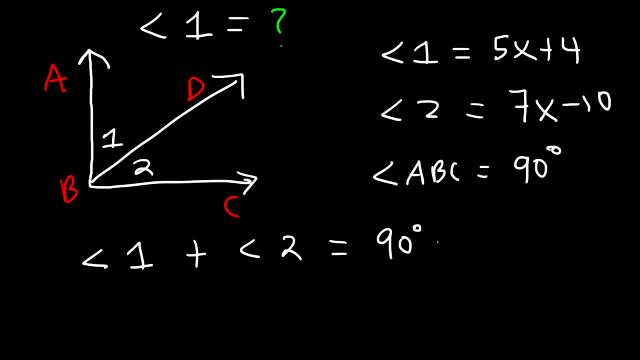 it's said that those angles are complementary angles. Supplementary angles add up to 180.. Now we can replace angle one with 5X plus four, because those two are equal to each other and angle two is and angle two is is 90.. 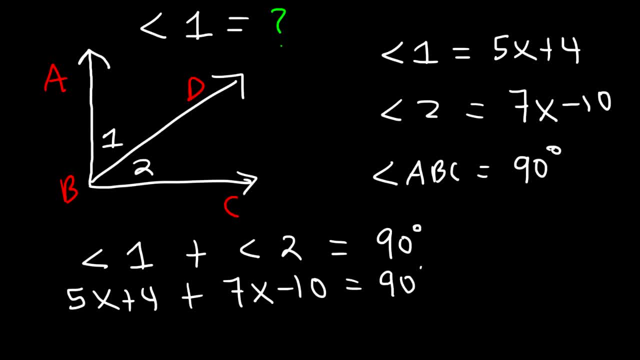 7x minus 10. so if we could find the value of X, we could find the measure of angle 1. once we have the value of X, all we need to do is plug it in to 5x plus 4 and that's going to give us the measure of angle 1. so let's simplify the 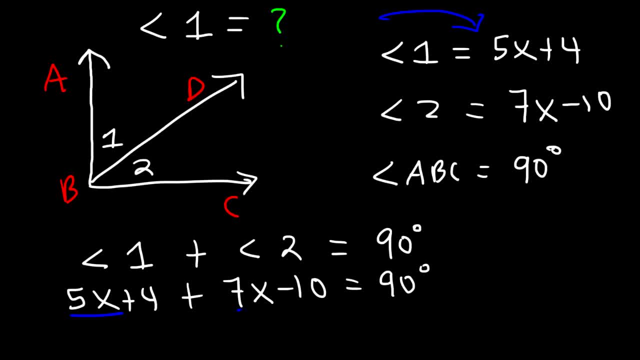 equation on the left side. let's combine like terms: 5x plus 7x is 12x, and 4 minus 10 is negative 6. so 12x minus 6 is equal to 90. so now what we're going to do is: 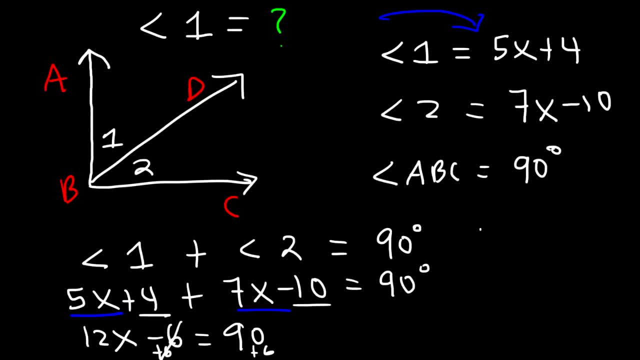 add 6 to both sides, so on the left side all we're going to have left over is 12x, on the right side, 90 plus 6, which is 96. so now what we need to do is divide both sides by 12. 12 goes into 96 8 times, so X is equal to 8. 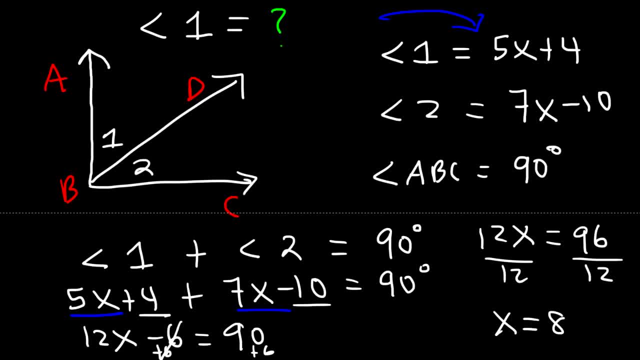 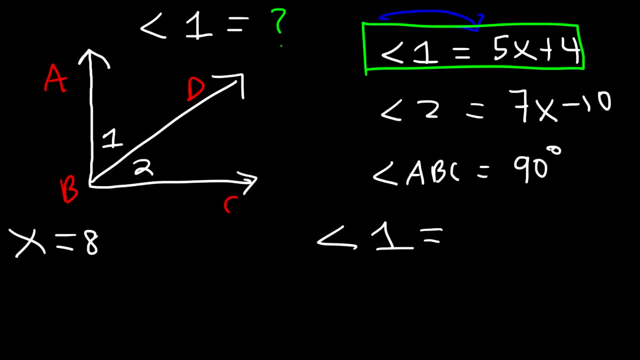 so now that we have the value of X, we could find the measure of angle 1. so let's replace angle 1- I mean X- with 8. so angle 1 is going to be 5 times 8 plus 4. 5 times 8 is 40, 40 plus 4 is 44. so the measure of angle 1: 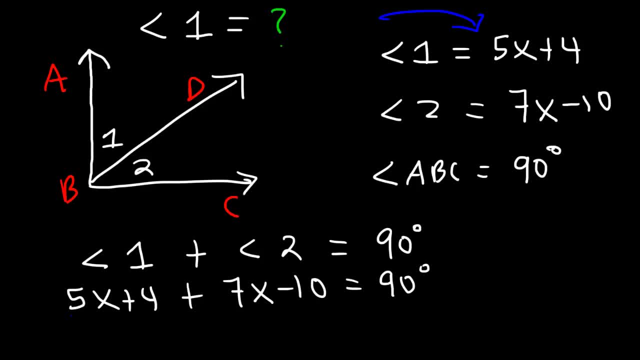 So let's simplify the equation. on the left side. Let's combine like terms: 5x plus 7x is 12x, and 4 minus 10 is negative 6.. So 12x minus 6 is equal to 90. so now what we're going to do is add 6 to both sides, so on. 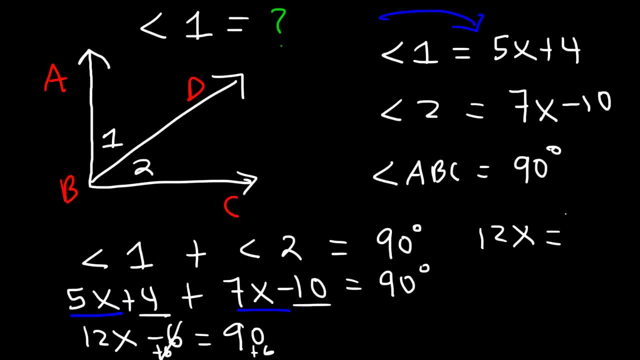 the left side. all we're going to have left over is 12x. on the right side, 90 plus 6, which is 96. so now what we need to do is divide both sides by 12. 12 goes into 96 eight times, so X is equal to 8. 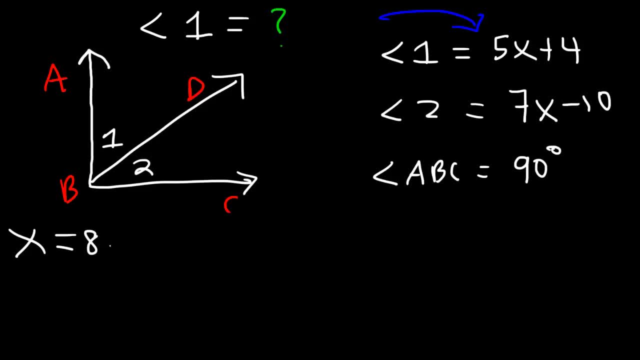 so now that we have the value of X, we could find a measure of angle one. so let's replace angle 1- I mean X- with 8. so angle 1 is going to be 5 times 8 plus 4. 5 times 8 is 40, 40 plus 4. 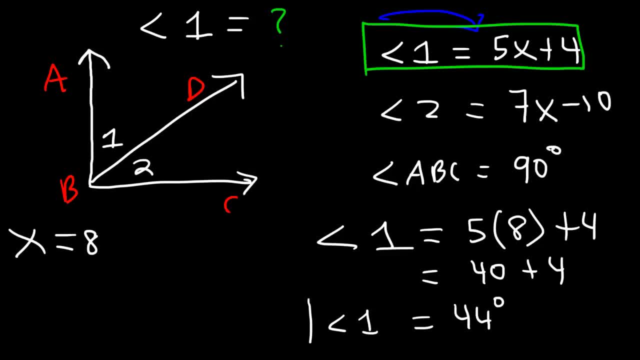 is 44. So the measure of angle 1 is 44 degrees. Now if we want to find the measure of angle 2, it's 90 minus 44. So it's 46 degrees. But the answer that we're looking for in this problem 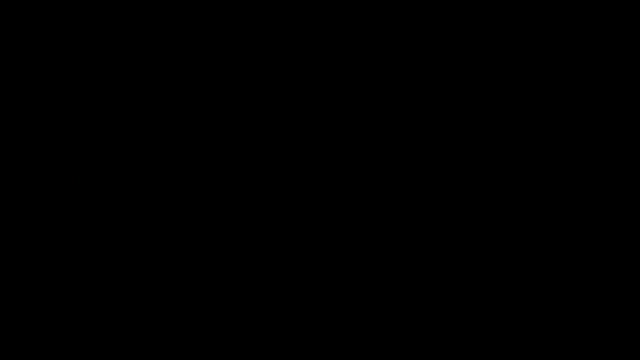 is the measure of angle 1, which is 44.. Now here's another example. So let's say this is A, B C. Let's say A B C is a straight line. Let's make this D and E And let's say angle E B C is equal to 70 degrees. 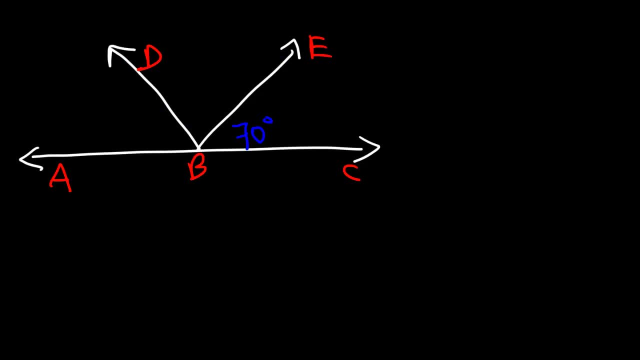 And angle D, B, E is equal to 70 degrees And angle D B E is equal to 70 degrees And angle D, let's say it's 60.. What is the measure of angle A, B, D? 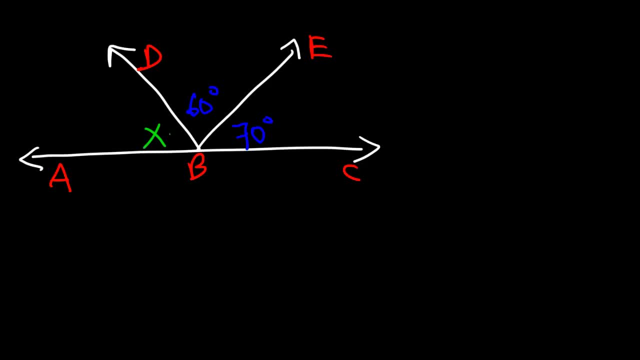 Let's call it X. Find the value of X in this example And remember: line A, B, C is a straight line, which means it forms a straight angle. Whenever you have a straight angle, the sum is 180 degrees. 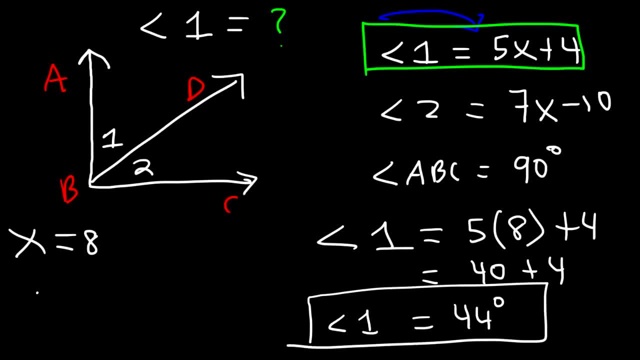 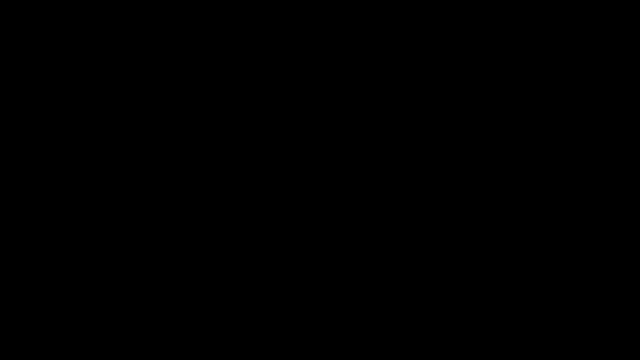 is 44 degrees. now if we want to find the measure of angle 2, it's 90 minus 44, so it's 46 degrees. but the answer that we're looking for in this problem is the measure of angle 1, which is 44. now here's another example. 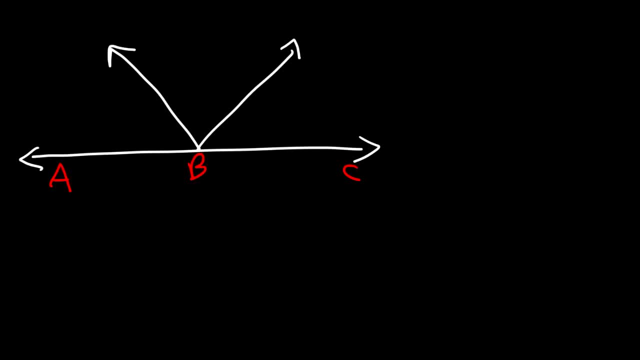 so let's say this is ABC. let's say ABC is a straight line. let's make this D and E, and let's say angle ABC is equal to 70 degrees and angle DBE let's say it's 60. what is the measure of angle ABD? let's 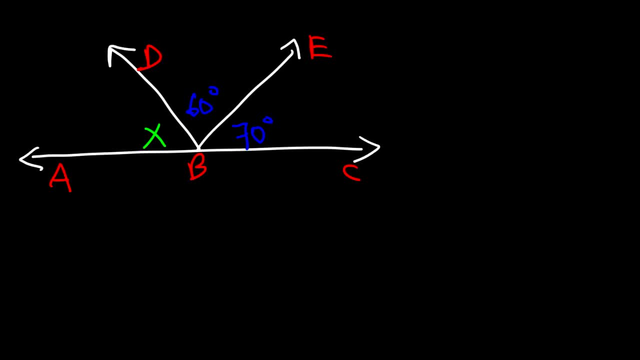 call it X, find the value of X, and it's right. you can write this into this example and remember: line ABC is a straight line, which means it forms a straight angle. whenever you have a straight angle, the sum is 180 degrees. so that means these three angles have to. 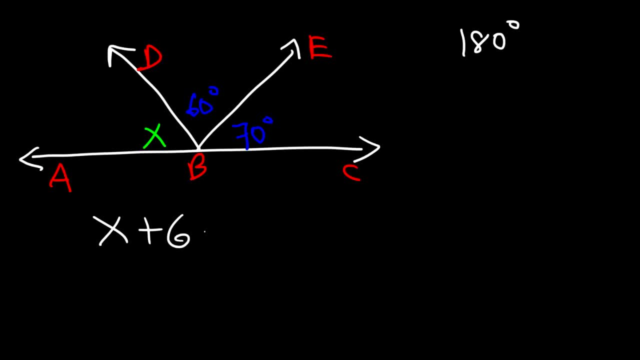 add up to 180 so we can write an equation: X plus 60 plus 70, you 60 plus 70 is 130.. And to find the value of X we need to subtract both sides by 130.. So 180 minus 130 is 50.. 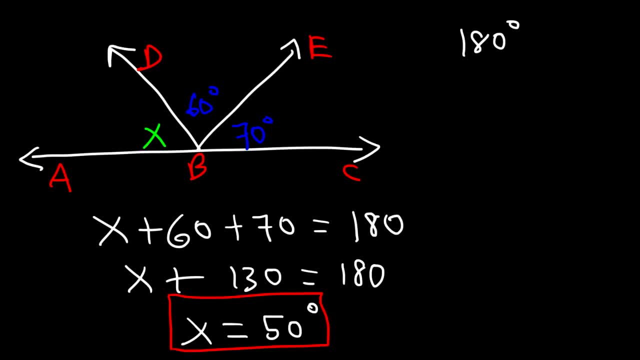 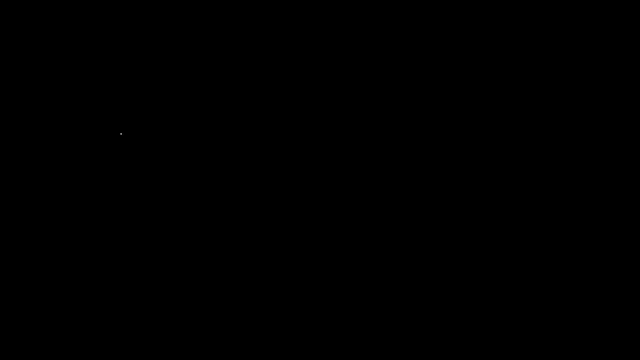 So that's the value of X, which is the measure of angle ABD, or you can call it angle DBA. So here's another example. Let's say this is line ABC, Let's call angle DBC angle 2, and ABD is going to be called angle 1.. 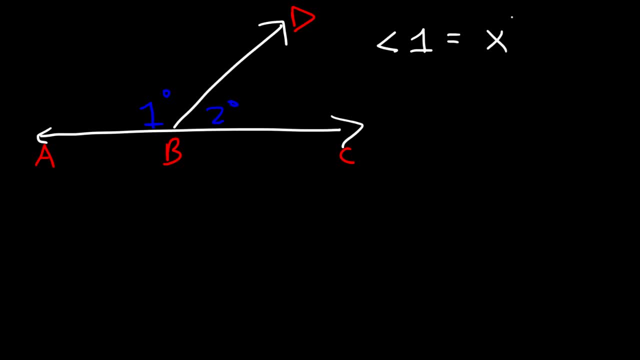 Now let's say that angle 1 is equal to X squared plus 16.. And angle 2 is 20X squared plus 16.. X minus 25.. And keep in mind, ABC is a straight line. What is the measure of angle 2?? 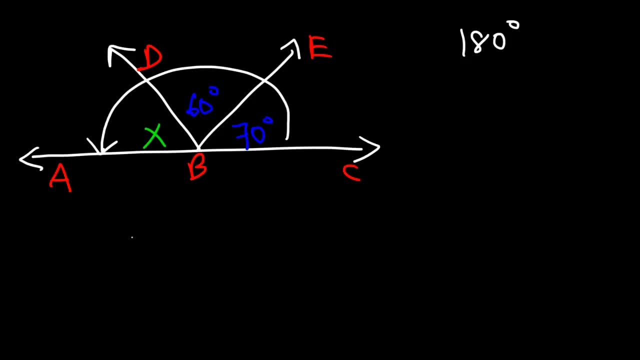 So that means these three angles have to add up to 180.. So we can write an equation: X plus 60 plus 70.. Now 60 plus 70 is 130.. And to find the value of X we need to subtract both sides by 130. 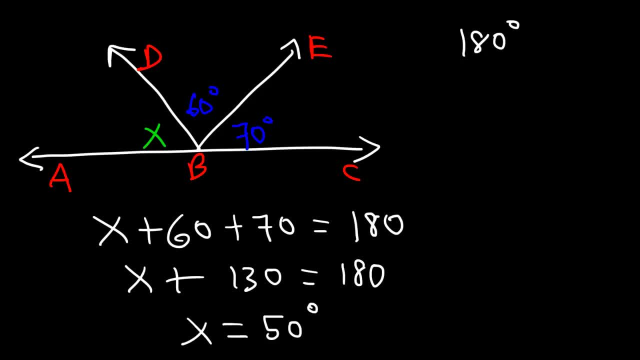 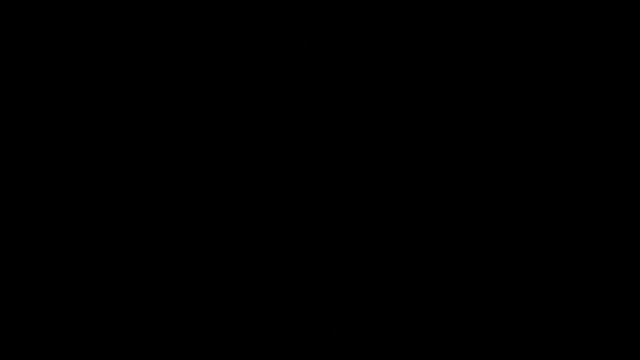 Or you can call it angle D, B A. So here's another example. Let's say this is line A, B C. Let's call angle D, B C angle 2.. And A, B, D is going to be called angle 1.. 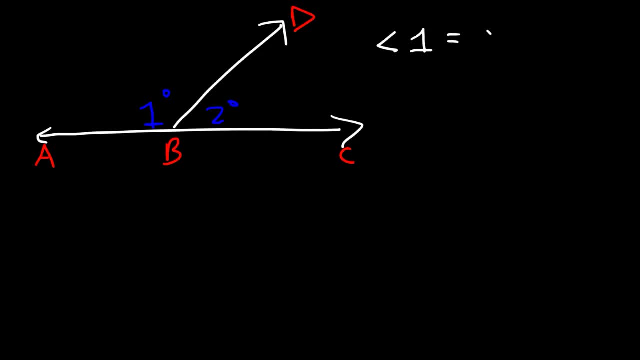 Now let's say that angle 1 is equal to X, B, D, or you can call it angle 1.. So angle 1 is equal to X squared plus 16. And angle 2 is 20X minus 25.. 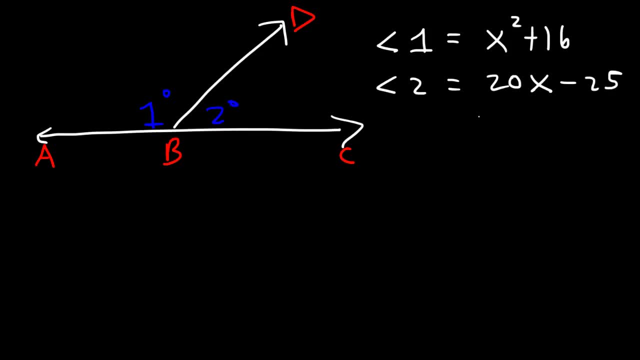 And keep in mind A, B, C is a straight line. What is the measure of angle 2?? Feel free to pause the video and try this problem Now. if A, B, C is a straight line, that means that angle 1 and angle 2. 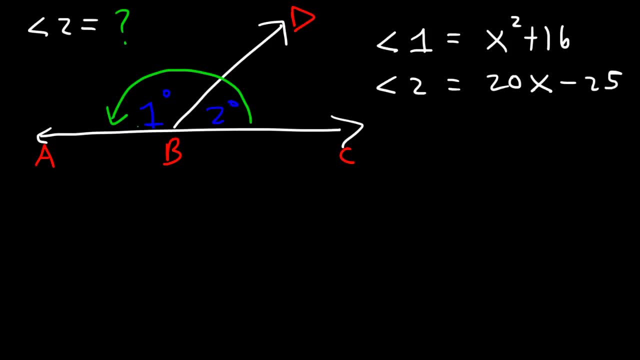 adds up to 180. Whenever you have 2, 2 angles that add up to 180, they're known as supplementary angles. So let's write an equation: Angle 1 plus angle 2 is equal to 180.. Now angle 1 is X squared plus 16.. 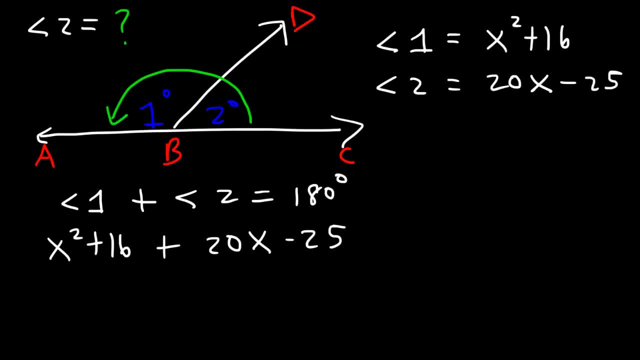 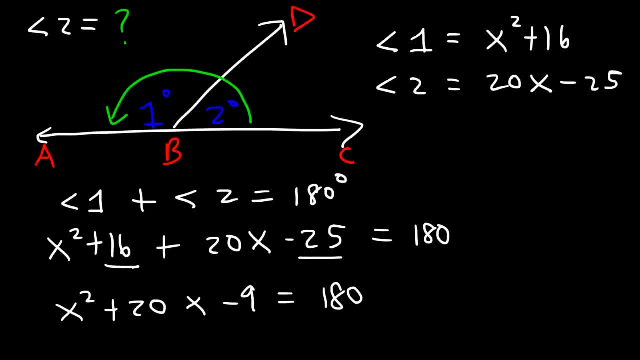 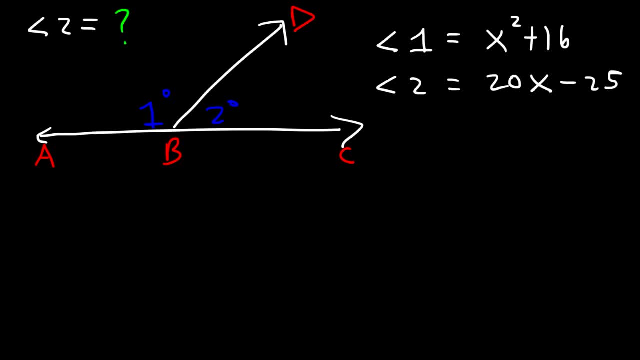 Feel free to pause the video and try this problem Now. if ABC is a straight line, that means that angle 1 and angle 2 adds up to 180.. Whenever you have two angles that add up to 180, they're known as supplementary angles. 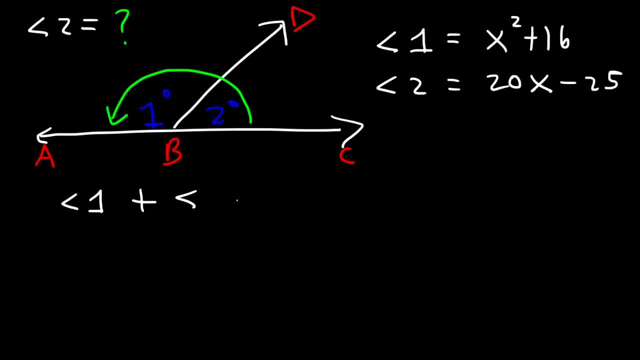 So let's write an equation. Let's write an equation: Angle 1 plus angle 2 is equal to 180.. Now angle 1 is X squared plus 16.. Angle 2 is 20X minus 25.. So now let's simplify the equation. 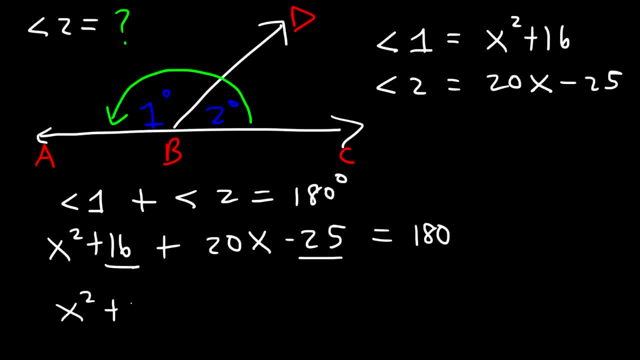 16 minus 25 is negative 9.. Now notice that we have a quadratic equation, Which means We need to take the 180,, move it to the left side and then to find the value of X, we can use the quadratic formula or we can factor. 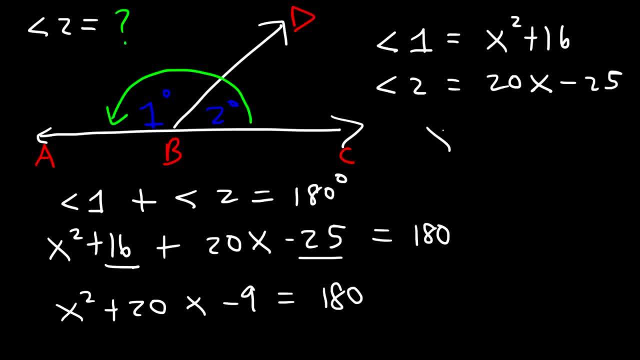 So if we subtract both sides by 180,, this is going to be X squared plus 20X minus 189, which is equal to 0.. In order to factor this trinomial We need to find two numbers. Okay, That multiply to negative 189, but add to positive 20.. 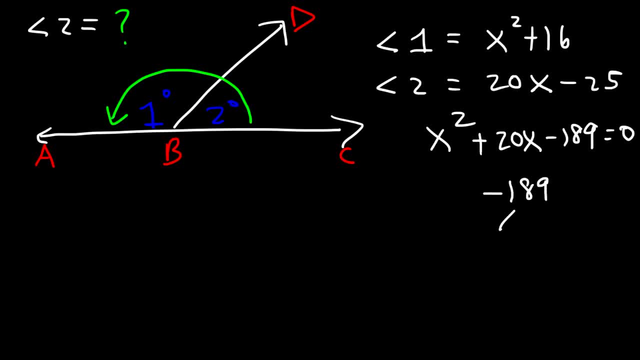 So what are those two numbers? It turns out that 189, it's not divisible by 2, but it is divisible by 3.. If you take in your calculator, if you type in 189 divided by 3,, you're going to get 63. 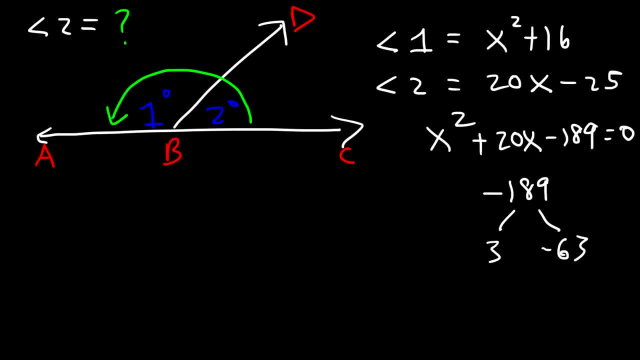 Now, 63 is 7 times 9.. Which means 189 is divisible by 7.. So we're going to multiply that, We're going to multiply that. We're going to multiply that. If you divide 189 by 7, you're going to get 27.. 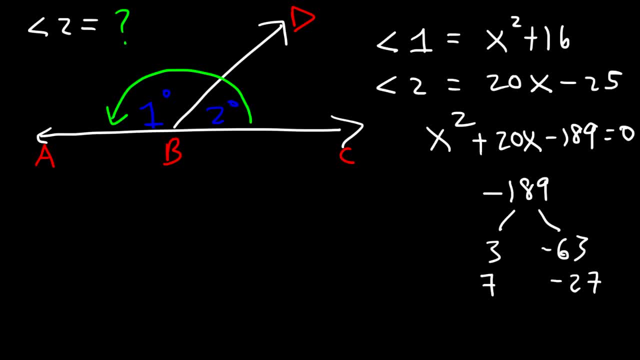 And notice that 7 and 27 differ by 20.. But 7 plus negative 27, that's negative 20, so we've got to reverse the sign. So what we want to use is negative 7 and positive 20.. 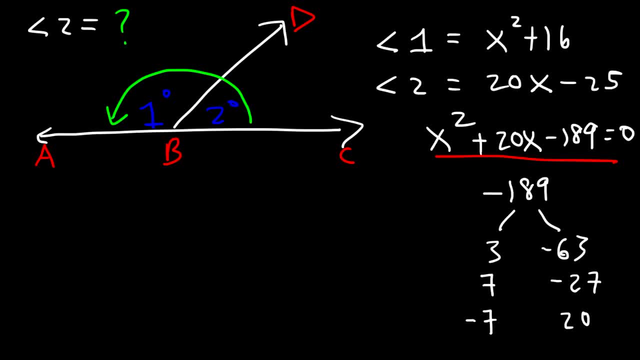 So therefore, to factor this expression, it's going to be X minus 7 times X plus 20.. And so that's equal to 0. Now We need to set each factor equal to 0.. Now, if X minus 7 is equal to 0, that means X is positive 7.. 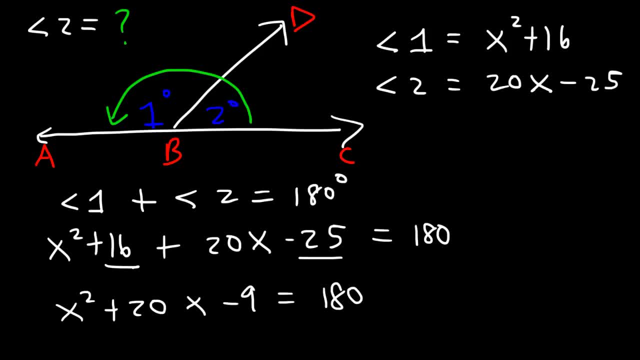 Which means we need to take the 180, move it to the left side and then to find the value of X, we can use the quadratic formula or we can factor. So if we subtract both sides by 180, this is gonna be X squared. 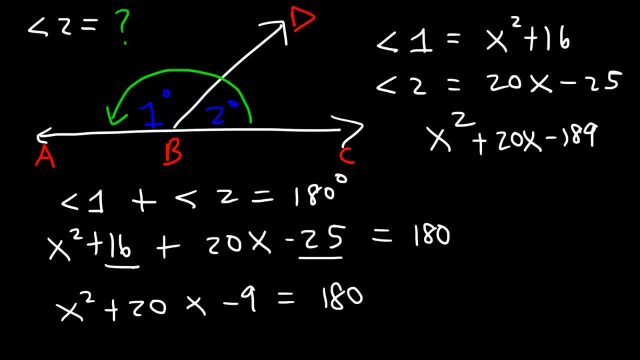 plus 20X minus 189,, which is equal to zero. In order to factor this trinomial, we need to find two numbers that multiply to negative 189, but add to positive 20.. So what are those two numbers? It turns out that 189, it's not divisible by 2,, but it is divisible by 3.. 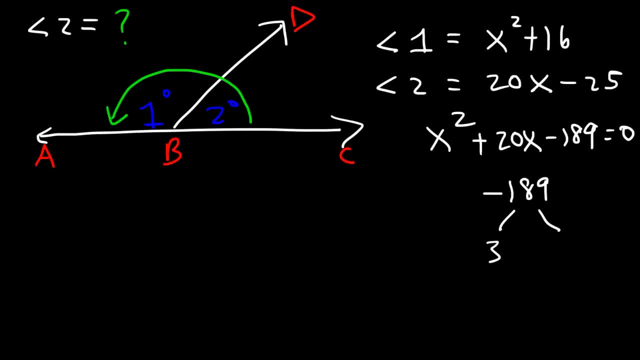 If you take in your calculator, if you type in 189 divided by 3, you're going to get 63. Now 63 is 7 times 9, which means 189 is divisible by 7.. If you divide 189 by 7, you're going to get 27.. 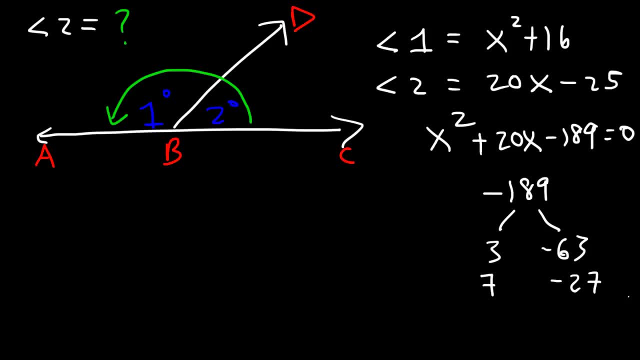 And notice that 7 and 27 differ by 20.. But 7 plus negative 27, that's negative 20, so we've got to reverse the sign. So what we want to use is negative 7 and positive 20.. 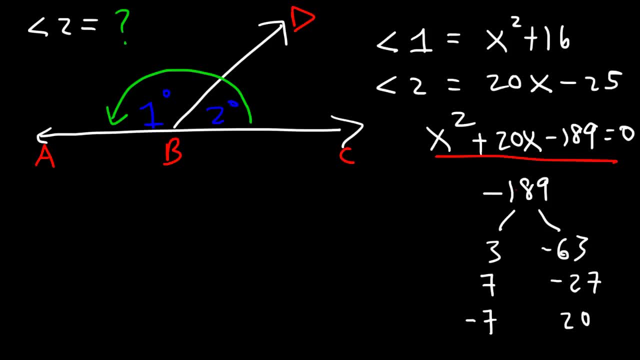 So, therefore, to factor this trinomial, we need to find two numbers that multiply to negative 20.. So, to factor this expression, it's going to be x minus 7 times x plus 20.. And so that's equal to 0.. 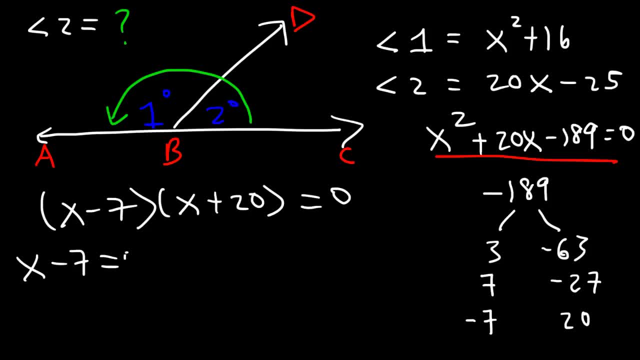 Now we need to set each factor equal to 0.. Now, if x minus 7 is equal to 0,, that means x is positive 7. And if x plus 20 is equal to 0,, that means x is negative 20.. 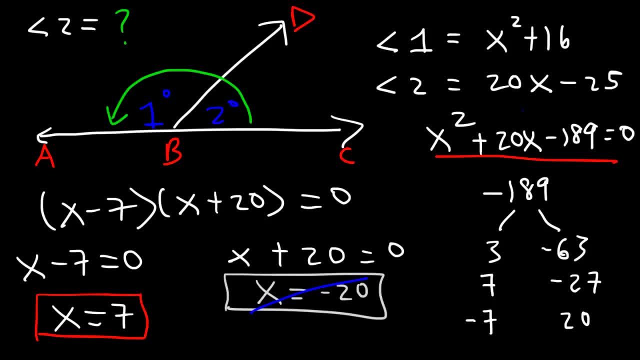 Now we're not going to use this answer, because if we plug in negative 20, we're going to get negative 20.. If we plug in negative 20 into angle 2, we're going to get a negative angle And that's not practical. 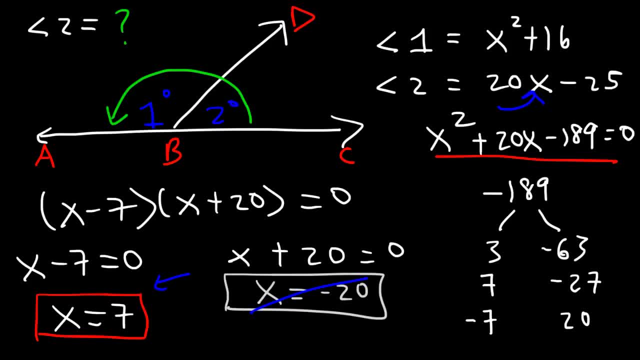 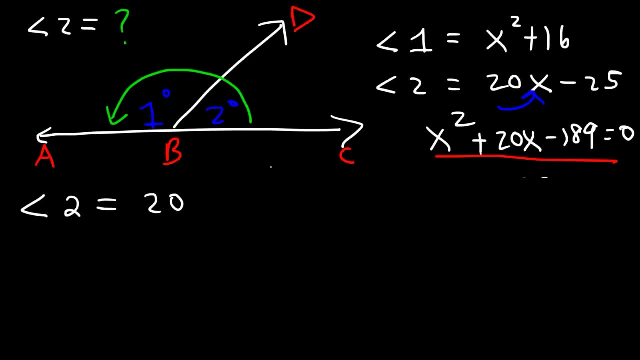 So therefore, x is equal to 7.. So now that we have the value of x, we can find the measure of angle 2.. So angle 2 is equal to 20x minus 25.. But let's replace x with 7..